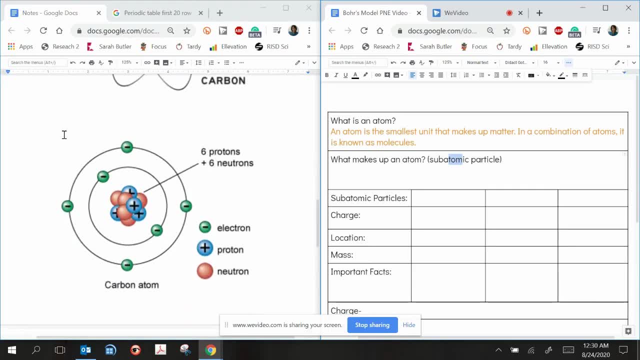 This atom and this atom models are the same, However. this is known as the Bohr's model, which is created by Niels Bohr. What he did is he fouled out the rings on the outside so we can count them easier. 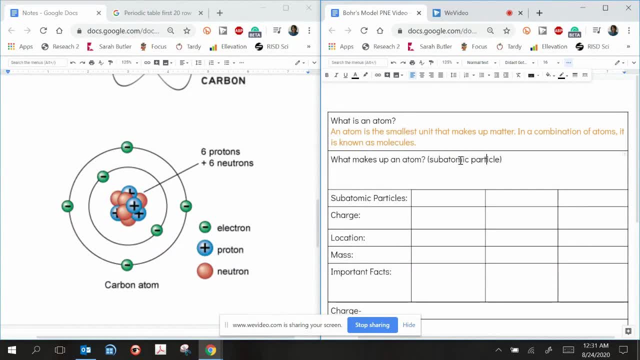 So what makes up an atom? Subatomic particle, Sub means parts, atomic means atoms. So what are the parts of an atom? Let's take a look. As you can see, the blue dot is representing the protons, The red dot is representing the belts. 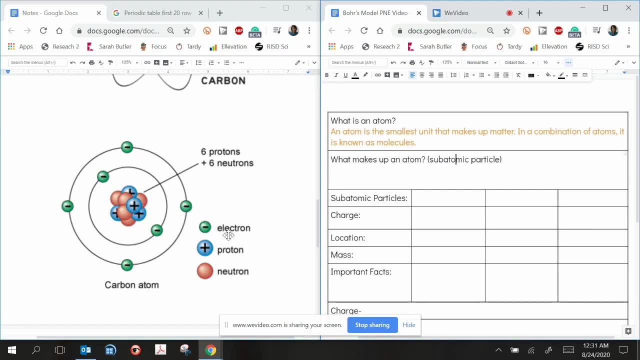 neutrons, and then the green dot is representing the electrons. So let's take some notes. What makes up an atom? Protons, neutrons and electrons. These are known as the subatomic particles, and you can also type them here. I'm using different colors to represent the diagram right here, so you know which one we're. 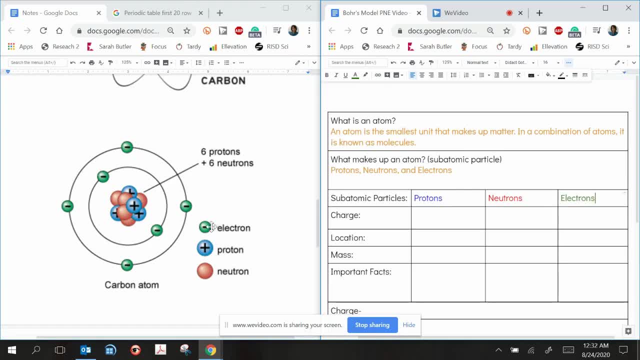 talking about. So let's take a look at the charge. The charge of a proton, as you can see, it says positive. Another way to think about it is you need to charge your battery on your phone. So the charge of a proton, as you can see, is positive. 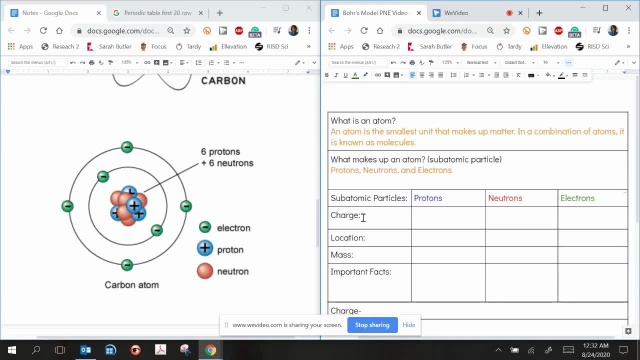 In a battery you have a positive AND and a negative AND. So for protons it is positive, which we use the plus sign to represent it. For neutrons it's neutral. Now it is not written here, but usually we use the zero sign to represent it. 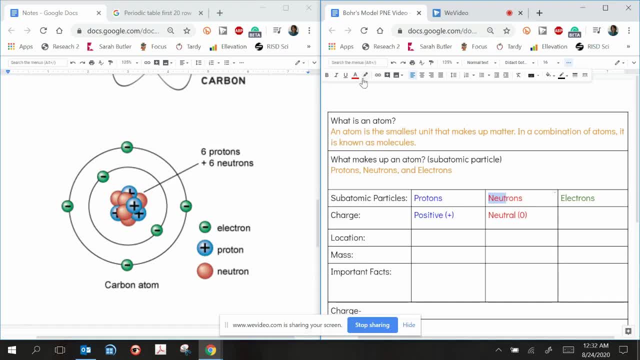 And an easier way for you to remember is neut. So you will always remember that neutrons are neutral, zero charge Location- So we just talked about it- is the center of the atom. What is it called again? Yes, the nucleus. 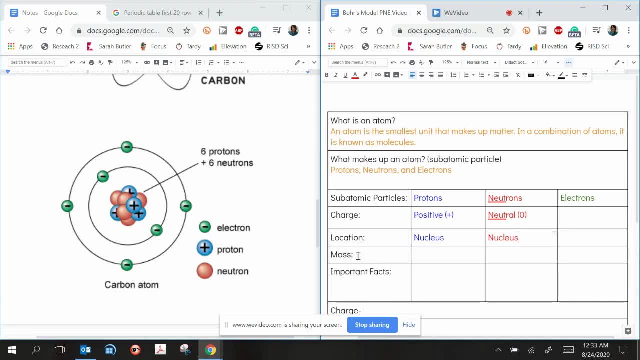 Now the mass. What does this term mean? Mass means weight without gravity. You can also think about how heavy it is, or the size of the subatomic particles. So, as you can see right here, the protons and neutrons are about the same size, And in here protons is one a-m-u, a mu. Now it stands for atomic mass. 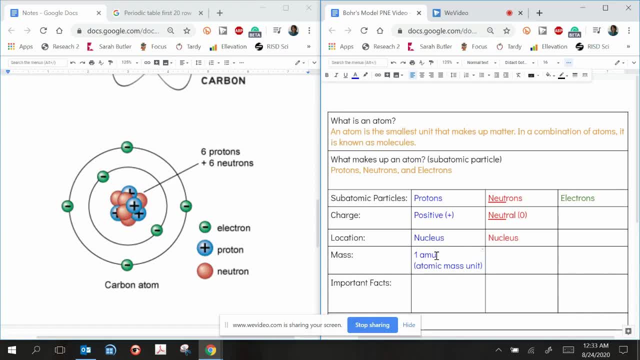 unit. This is just a weight unit, kind of like pounds, but only for atoms, Because if we use pounds then the number is going to be very, very, very, very small. So that's why we create a unit: just to measure how heavy it is for each subatomic particle within an atom And for neutrons. 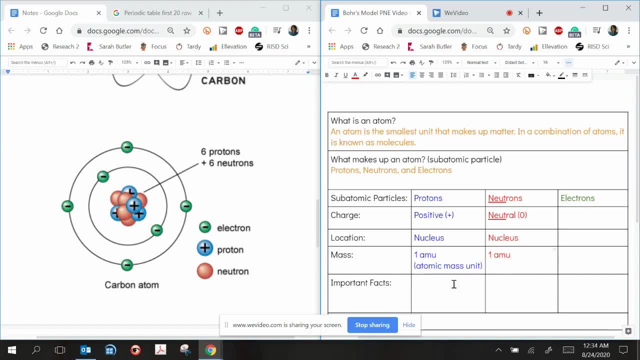 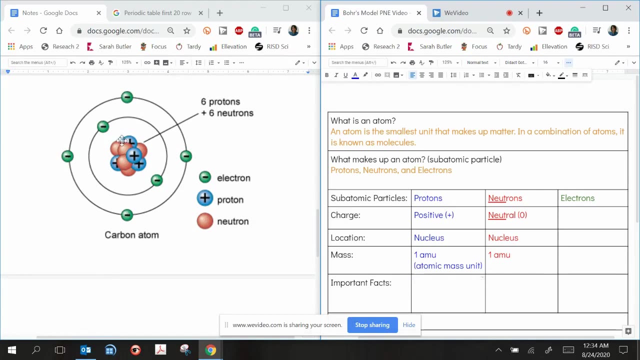 it is also the same one a-m-u. Now, important facts about protons. Protons is very, very special. So if you take a look at it right here, the carbon atoms has six protons. I know you only see four, but some of them are. 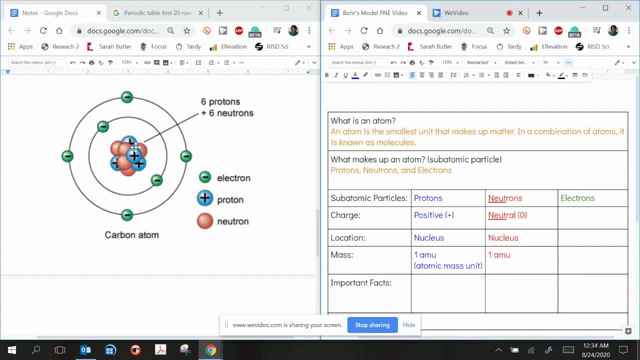 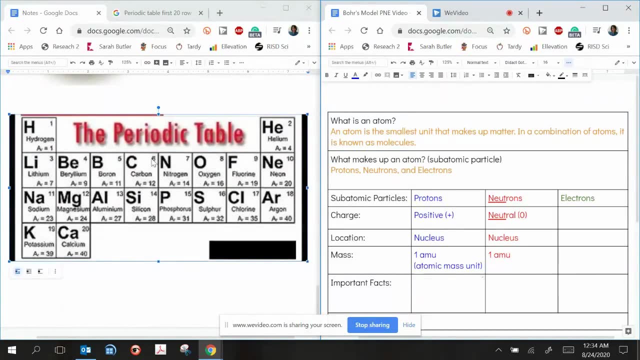 hiding behind the back. Okay, so six protons, And then the red ones are six neutrons. That's the protons. If you look on the periodic table, this number on the top right here, that is the ID number, okay, the identification number for carbon. So this number is kind of like. 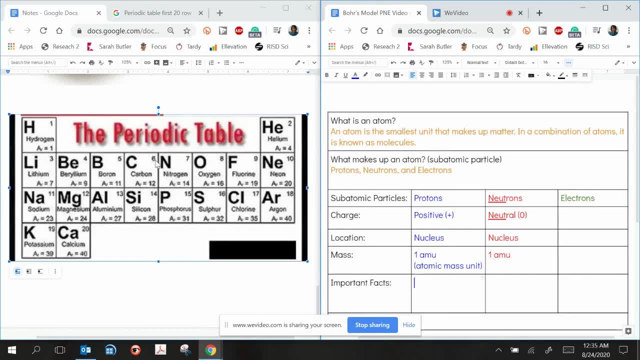 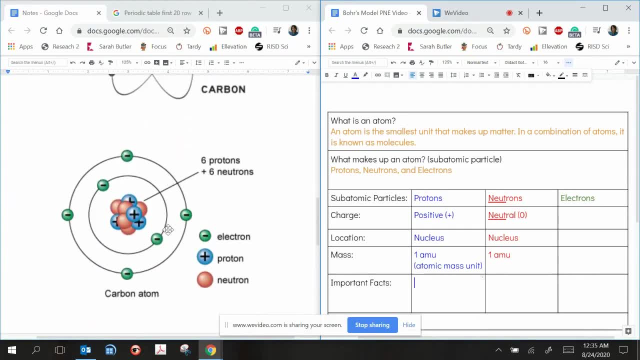 carbon student ID that once you call out it is six. we know that it is carbon. So it's based on the positive sign that tells us what element or what atom it is on the periodic table. So you can say identification or ID. You see, your ID card is the abbreviation of identification, is the protons.